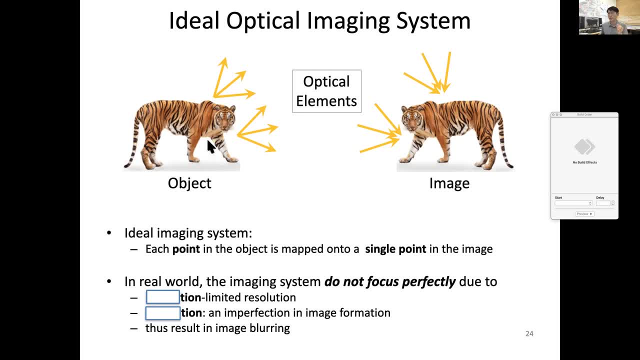 So ideal imaging system means each point in the object should be mapped onto a single point in the image. The question is the fidelity or the size of this infinitesimal point can become again infinitesimal Point, which means by infinitesimal resolution. So currently you can think of, let's say these are objects are composed of molecules, and molecules composed of atom, atom composed of, like nucleus and electron. 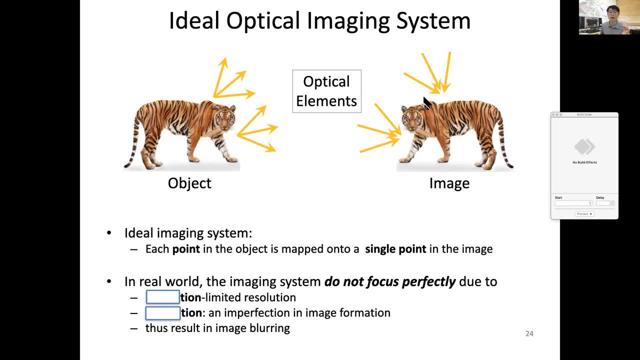 Yeah, those are objects. If you can map those one by one, you can have almost infinity of resolution. Why That is not possible? This is not possible. This is very important for whoever deals with an imaging system. Talk about it. That's about resolution. 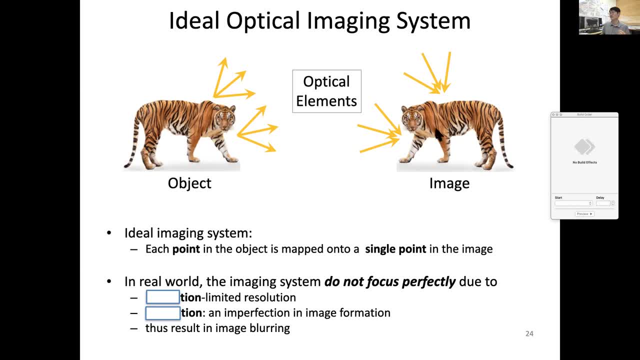 So in the real world, the imaging system actually does not focus perfectly. That's a problem, And we have to know where comes this limitation, What do we, how we can overcome this limitation. Okay, So first of all, as I said, geometric optics. 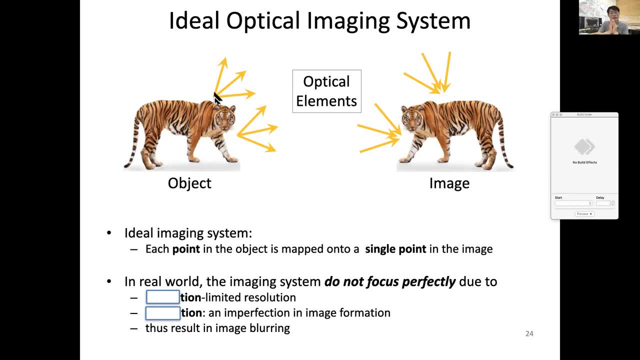 we talk about it like the one with the interface and lens. that is very ideal, So it doesn't show anything wrong and anything which degrades the resolution of optical system. But remember that the light we are dealing with has a duality. It can behave like particle light. 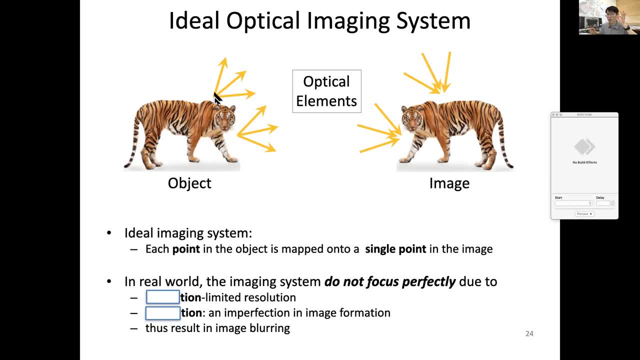 It can behave like a wave. Remember all the waves having a property when it interacts with an object, It should, It should Diffract or bending property. So, in fact, why we cannot get infinite, infinite amount of resolution by this optical element is first: 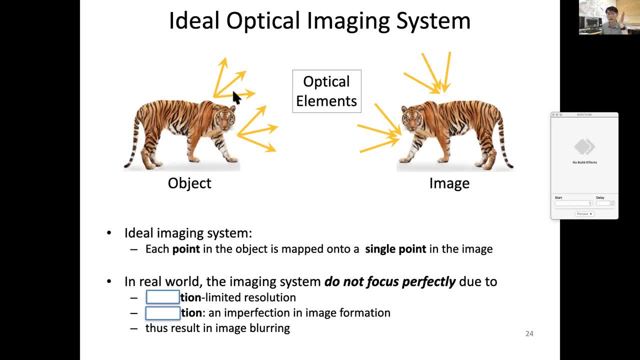 We are using light as a medium and light as a wave. It has a projects, a wave property, And when they deal with optical elements, these optical elements are finite, So it's a finite object. The wave would be défractive. 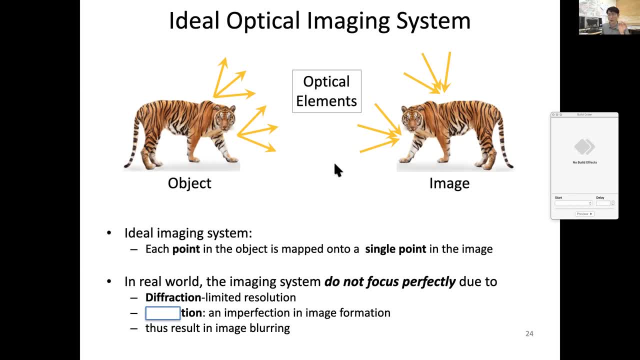 be diffracted somehow- And that is a fundamental issue of optical imaging system- by using light which has a wave-like phenomenon. Because of that there's a fundamental limitation of resolution. So the resolution really depends on the wave property of light, which is wavelength lambda. 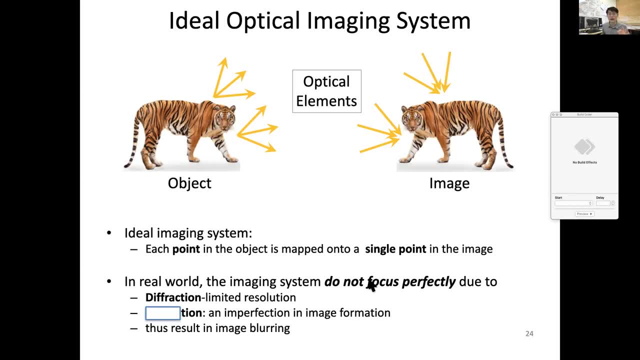 So remember, that's the key issue, that why we cannot focus perfectly. And, of course, when you generate this optical imaging system, what happens is you cannot align it totally perfect. And also the lens. over there we manufacture the lens, and the lens is not usually. 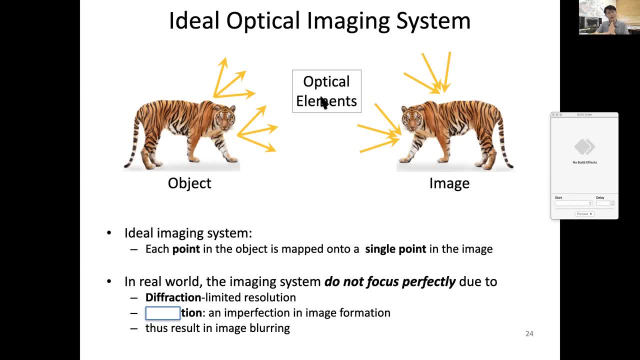 perfect lens. The easy way to manufacture a lens is making the surface as a sphere, The spherical way. So spherical lens we call, or convex lens, And that lens. if you use a geometric optics you realize the rays will not be perfectly focused down because the surface of the lens 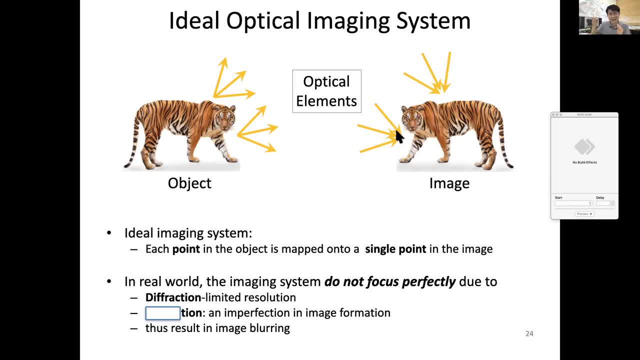 what we make. a spherical shape is not in fact ideal. So those imperfections in the information we call aperture, In Korea it's called sutra, So aberration can contain many aspects, but these two are the major cause of why we cannot have, let's say, one nanometer resolution, one Armstrong resolution. 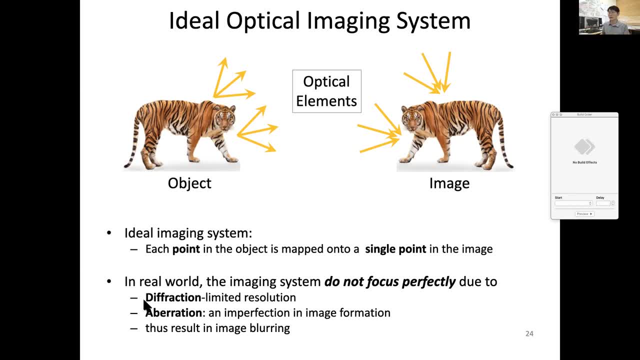 with an optical microscope. So this is something we want to have a fundamental here. a fundamental limit is, of course, diffraction limit, Because aberration- somehow if you are using poor optics you can use more expensive- or optics If it's a spherical aberration. 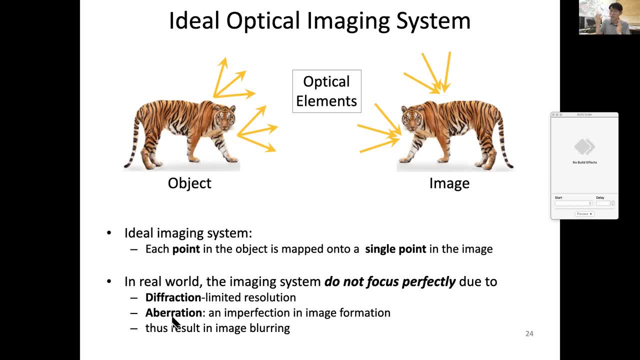 you can buy a spherical lens, which is much more expensive, So you can actually reduce this aberration. But somehow diffraction limit means the light is bending when it interacts with an optical element, And that is a fundamental wave nature of light. So it's kind of hard to overcome. So it's a fundamental wave nature of light, So it's kind of hard to overcome.